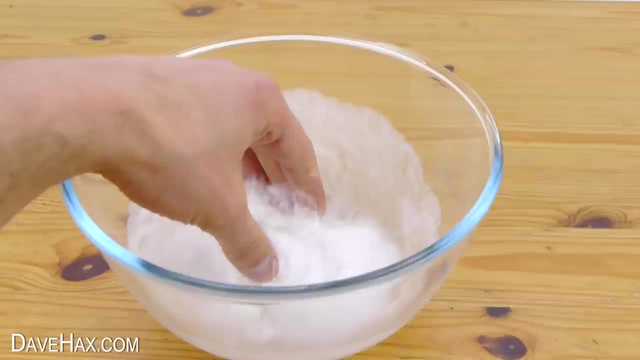 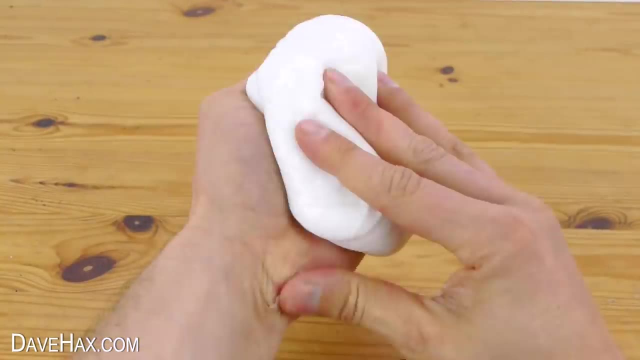 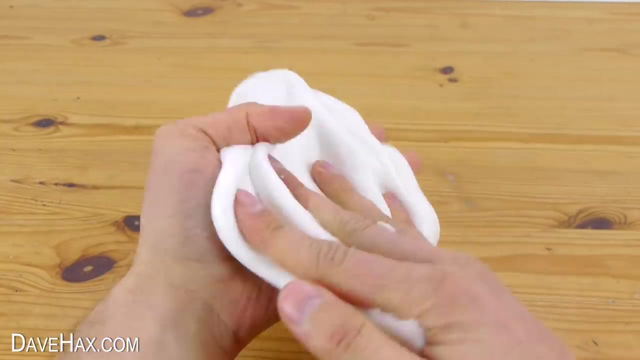 Keep on mixing it and after a while, you can use your hands to mold it all together. Keep on going and you should end up with a nice ball of slime like this. Pretty cool, huh. It's stretchy and slimy and really fun to play with. 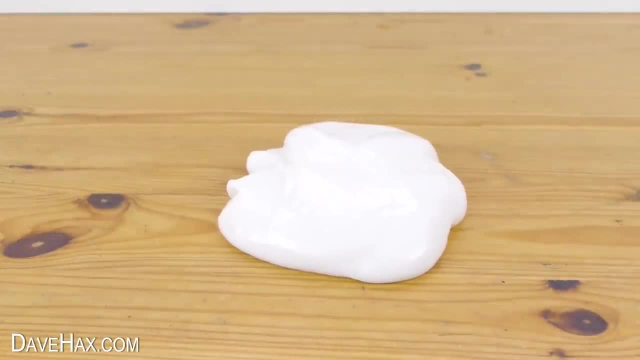 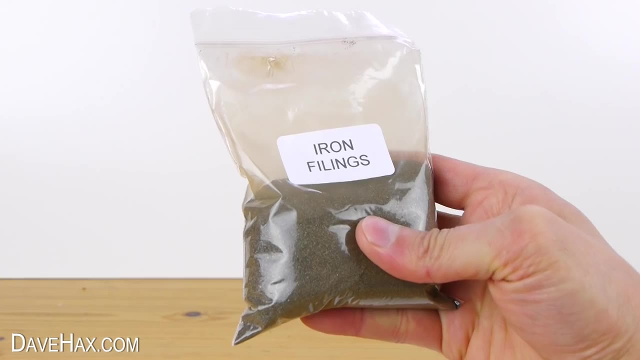 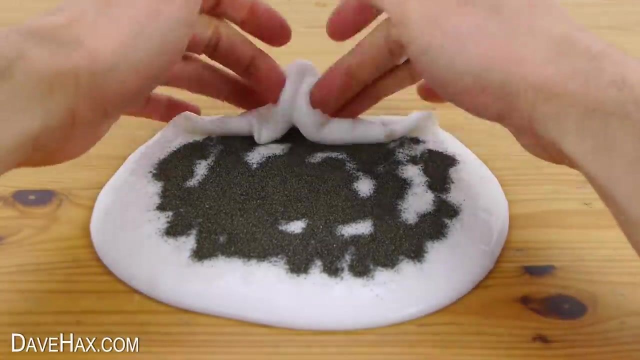 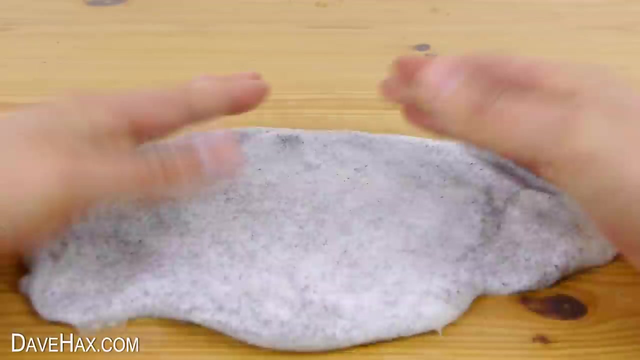 You can put it on the table and watch it melt into a blob. To make it magnetic, we're going to add some iron filings. Pour some onto the slime and carefully work it into the mixture. I'm adding a little bit more. 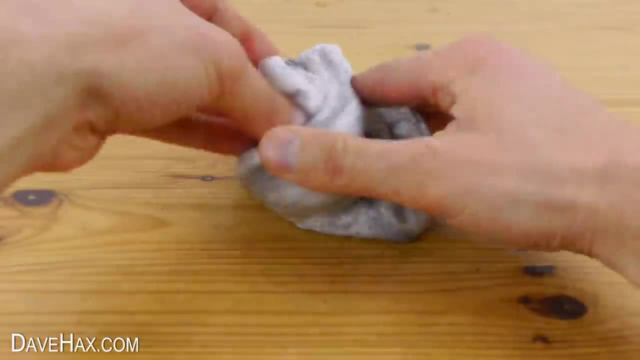 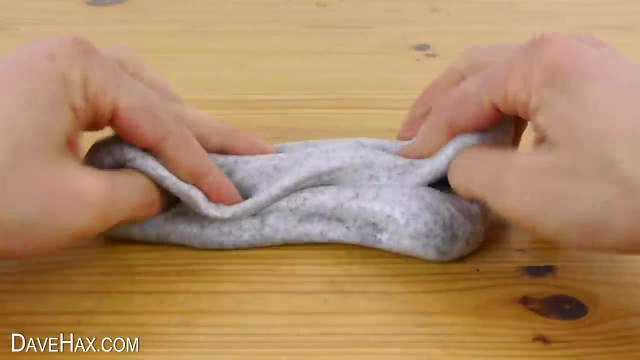 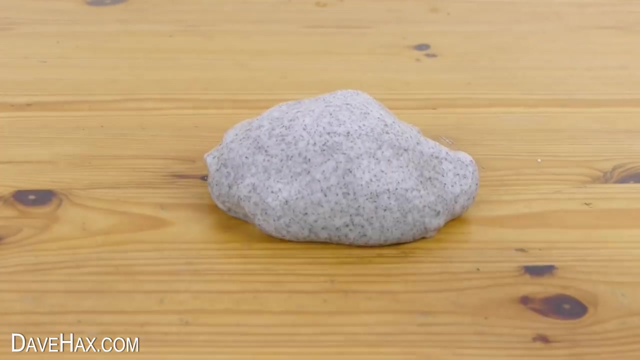 and really folding it in. You need to make sure there's no pockets of filings like this which haven't been mixed in. So keep on going And when it's ready, you should have a light grey slime. Now, if we take a magnet, 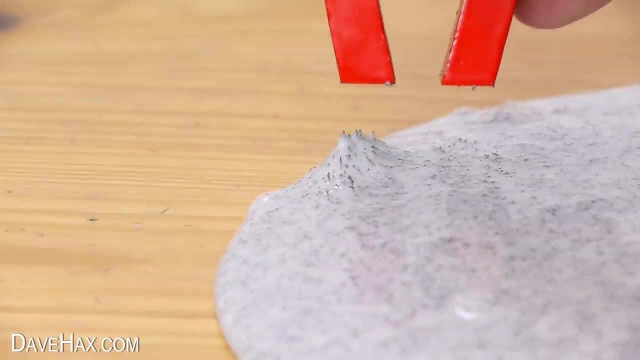 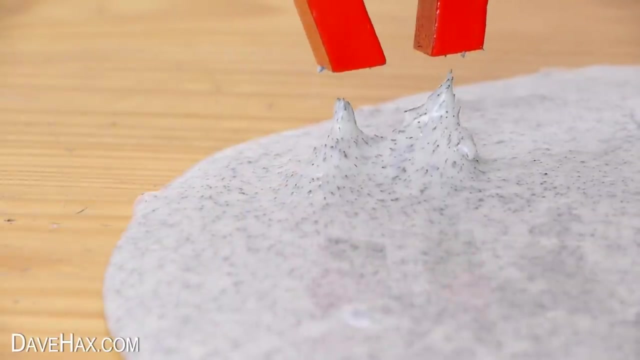 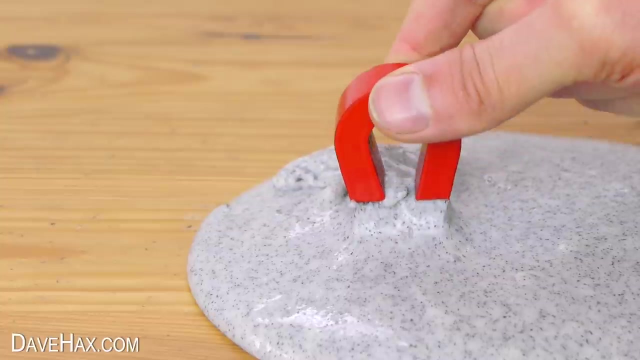 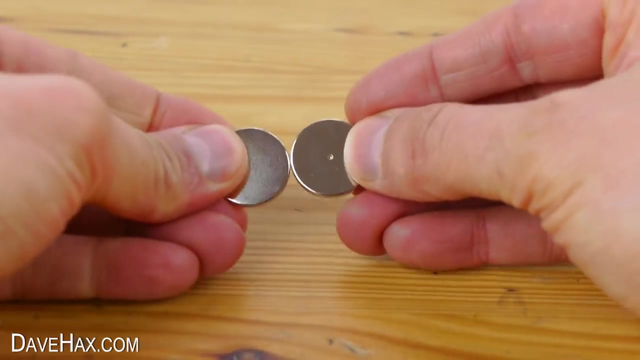 and hold it close by you can see how it reacts. The slime's attracted to the magnet and you can make it move. You've got to be quick or it'll stick to the magnet. These neodymium magnets are really powerful. 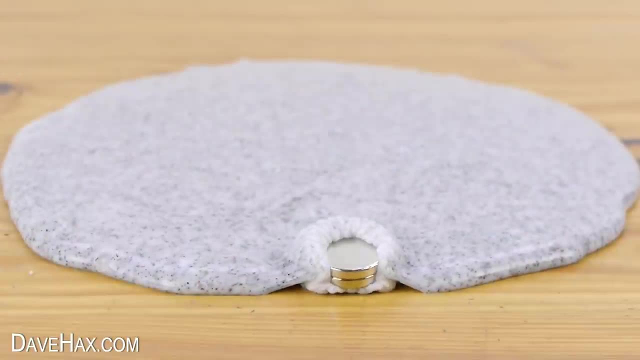 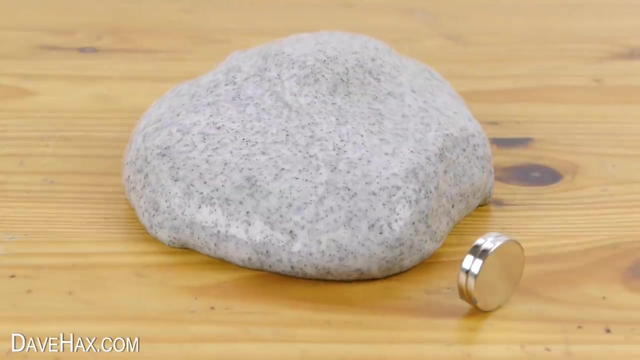 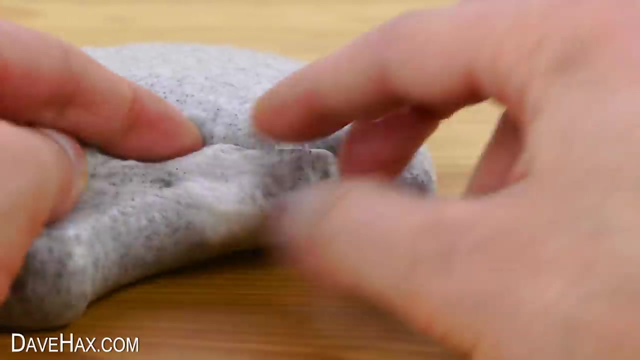 And you can watch what happens when they get stuck into the slime. Pretty cool, huh? I have speeded up some of the footage so it's quicker to watch. It can be difficult to get the slime and the iron filings back off the magnet. 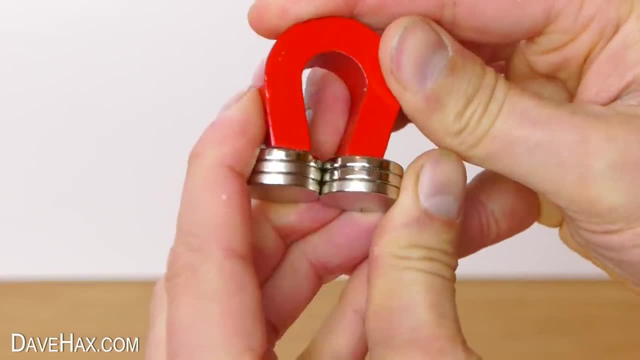 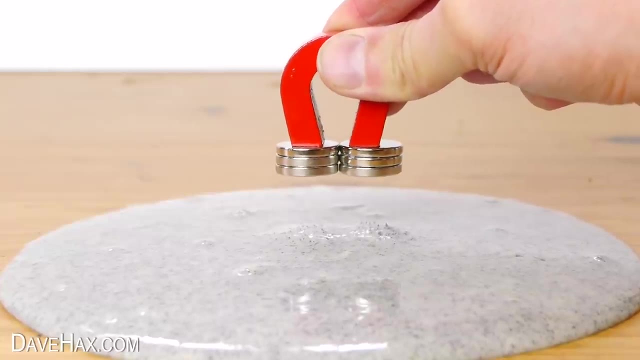 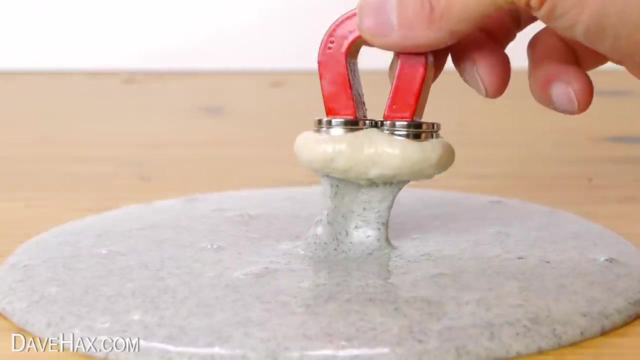 You can stack magnets to make them stronger and watch what happens as the slime jumps up and wraps itself around. And if you really want to see the fun, you can check out our list of how it works. And now we're ready to do some more. 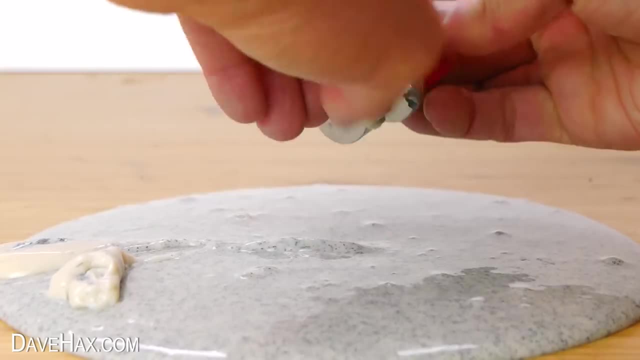 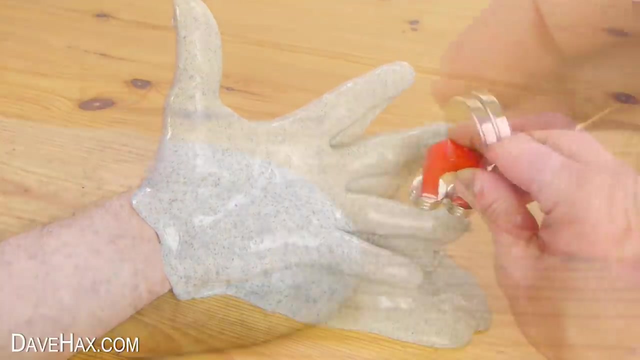 You can pick up the mat, make the home-69, and you can get in the motorhome. It's great fun to play around with and watch it all move. And I have made it a bit softer, so maybe you want to go a little faster.